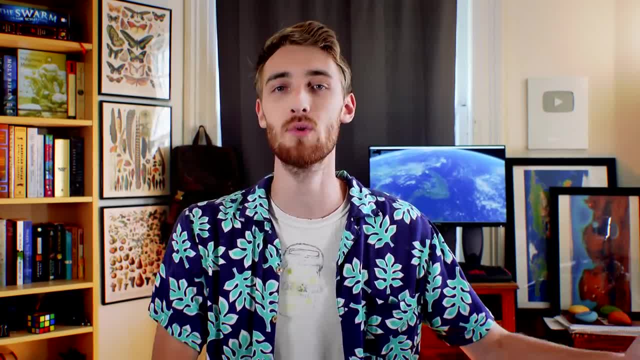 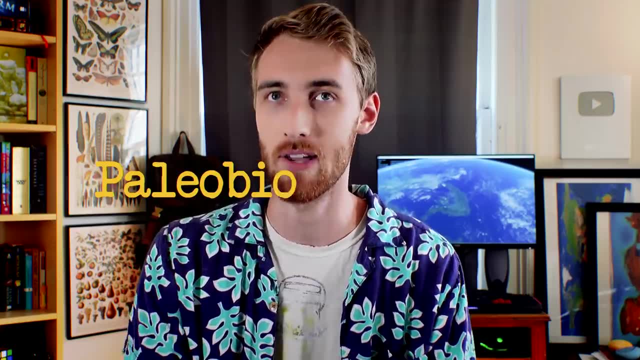 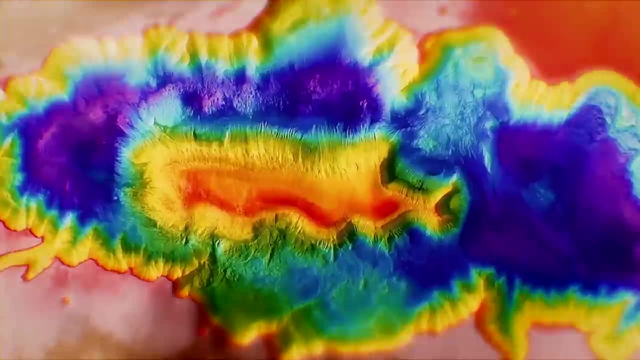 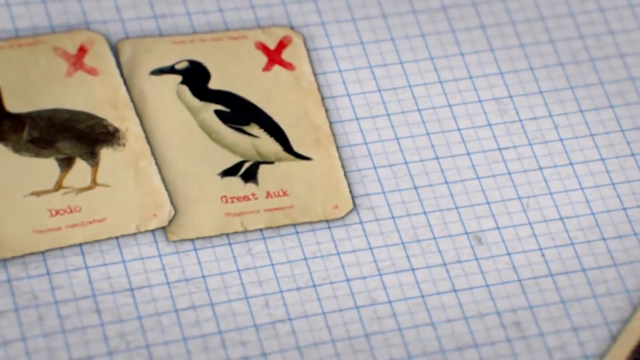 it's time to apply what we've been learning to a whole new cast of animals and see what the evolutionary laboratories that are islands cooked up in the way of paleo biogeography. Unlike the last two videos, this time we won't be starting by looking at a location. 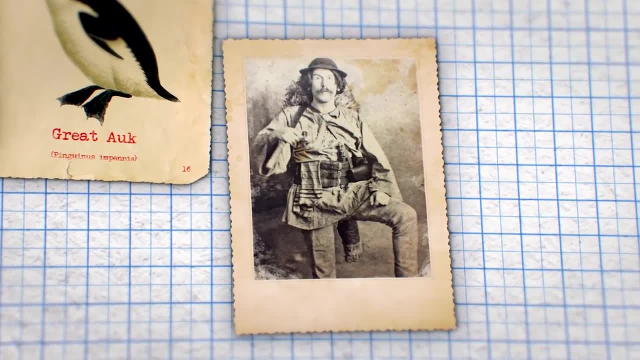 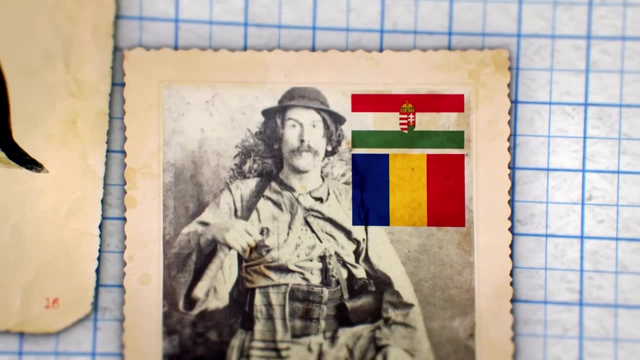 but rather today, our story begins with a person. This is Franz Nupška, a paleontologist from what used to be Hungary, but is now Romania, Despite being born to an aristocratic family. if you couldn't tell by the picture, 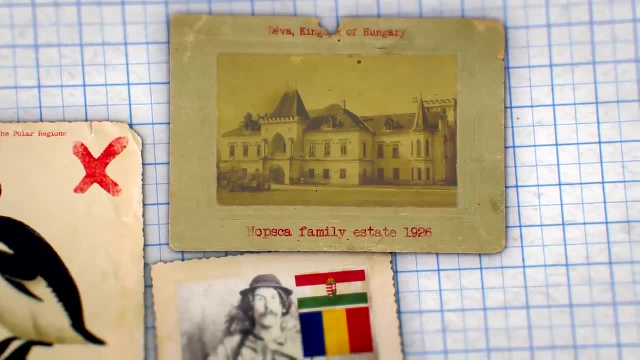 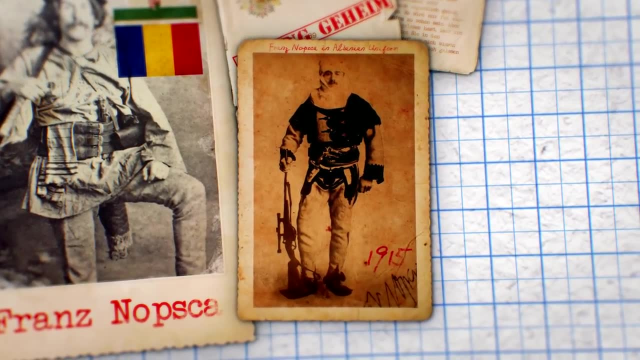 this guy had a pretty wild life, whose escapades include serving as a spy for Austria-Hungary, twice leading a band of freedom fighters against the Ottomans, trying to become the king of Albania, and being the first person to ever hijack a plane. 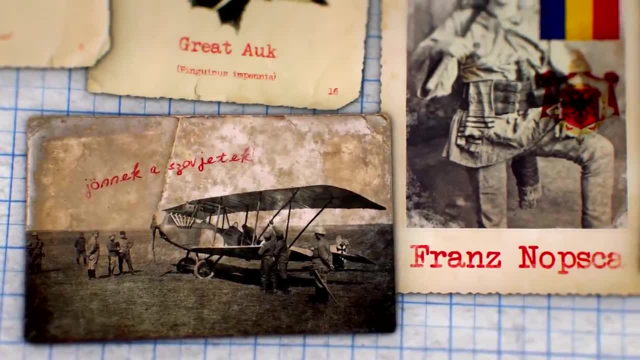 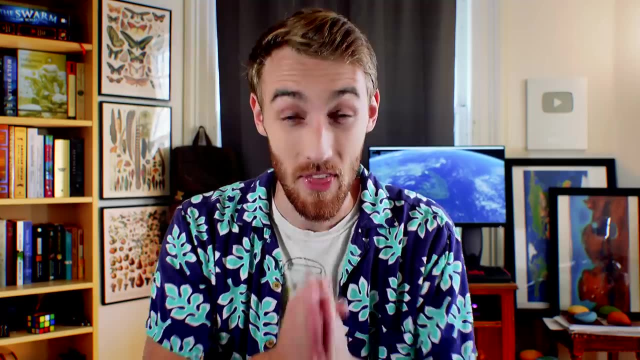 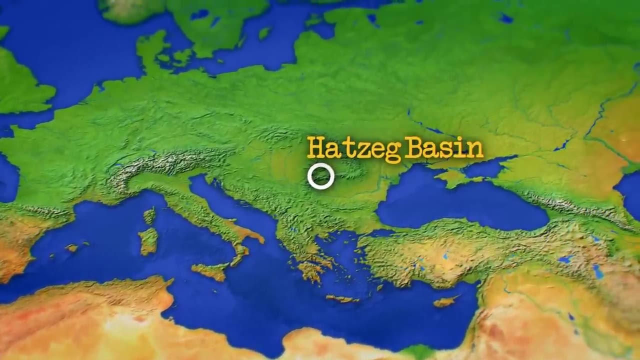 But somehow, in the midst of all this, Nupška also managed to conduct several extensive paleontological digs in and around his home within the Transylvanian Alps. That's the part we're interested in today, Specifically the digs that took place here within what's known as the Hatzeg Basin. 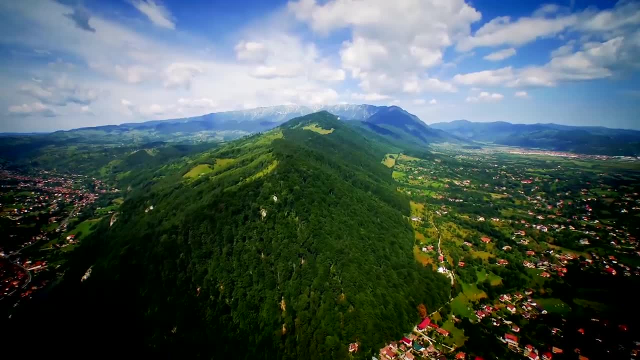 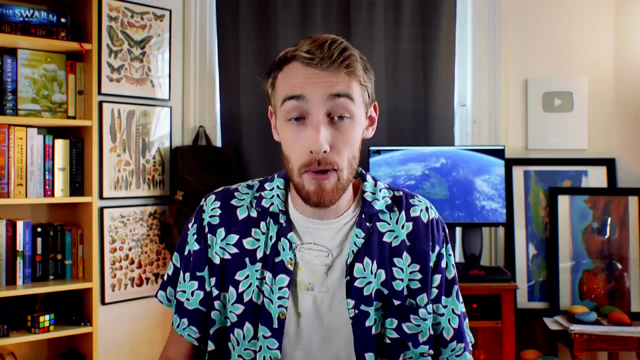 near the village of you guessed it- Hatzeg. Within the rock formations of this basin were numerous dinosaur remains, all dating back to roughly 70 million years ago. But what Nupška found here was at first disappointing. 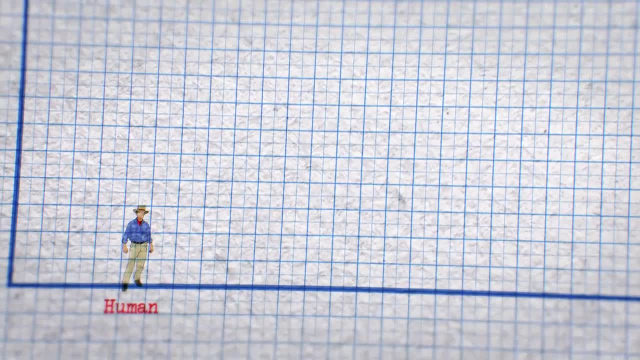 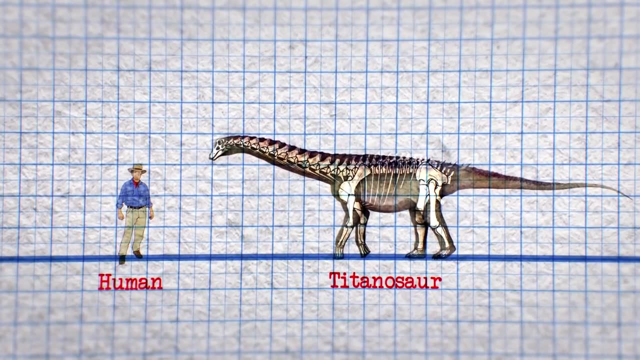 For example, the largest specimen he managed to uncover looked to be a sauropod, though based on its skeletal structure. not any regular sauropod, but rather a member of the titanosaurs, a clade of sauropods known to have grown. 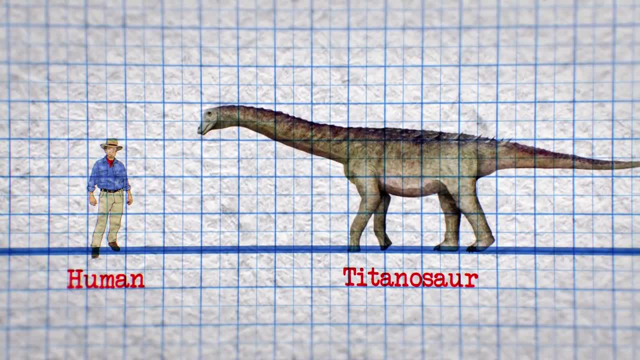 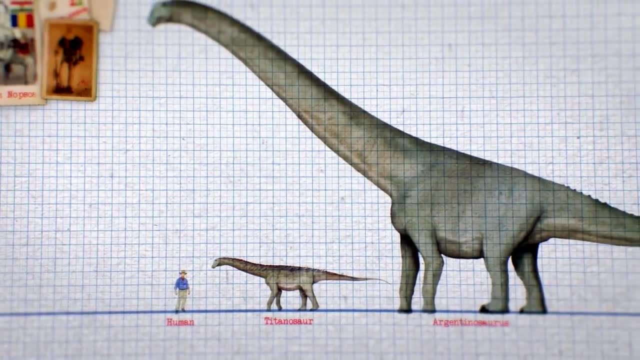 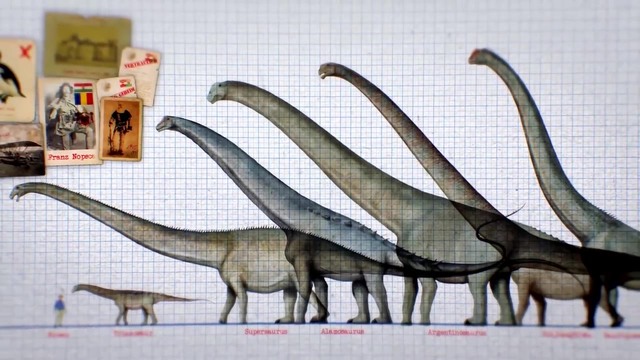 bigger than any other animal the planet has ever seen. The biggest titanosaur is thought to have been Argentinosaurus, which measured potentially over 35 meters long and 15 meters tall, though there were plenty of other titanosaurs that could have rivaled it. 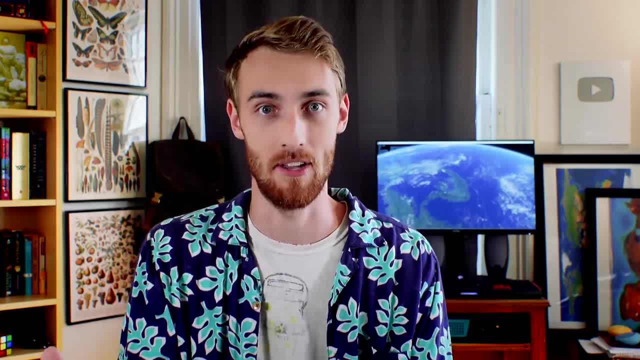 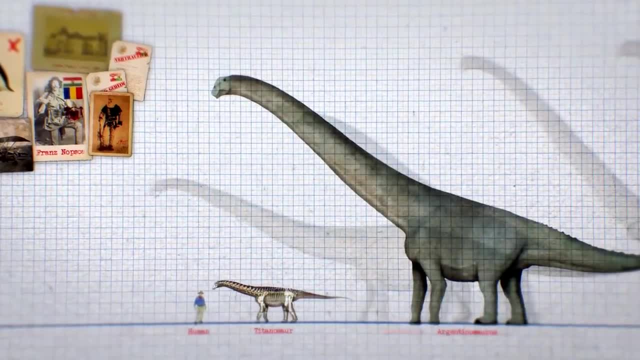 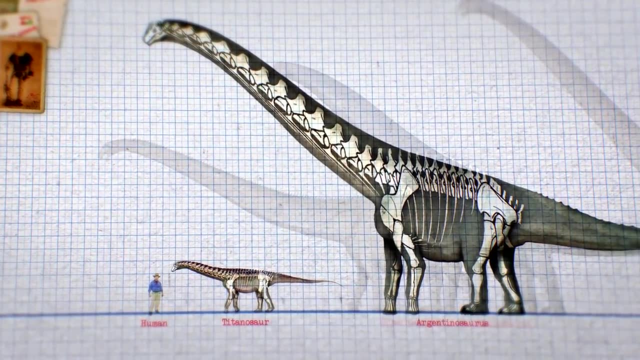 Or in other words, these things were typically ginormous, But the titanosaur that Nupška discovered was much less impressive. Despite having the same bone structure as a regular titanosaur, when all put together, Nupška's findings would have stood only 6 meters long and probably less than 2 meters tall. 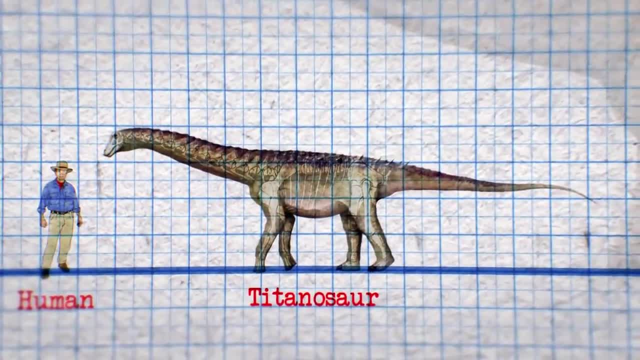 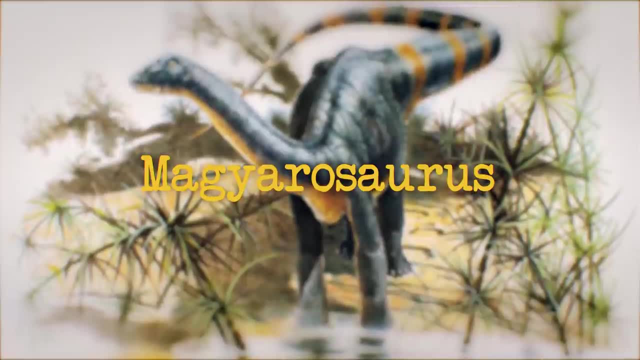 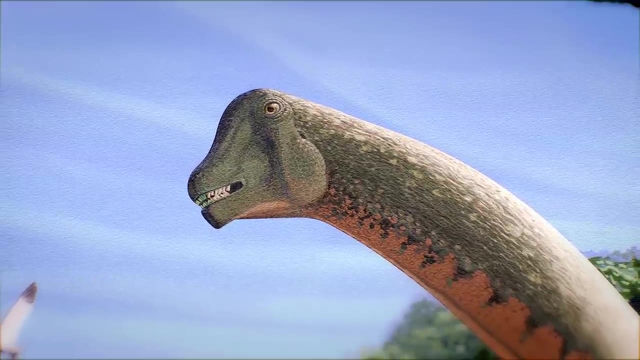 By all definitions, this was a puny specimen compared to its relatives Named after its discoverer's homeland. the Magyarosaurus for a while represented an oddity in the paleontological record. Most professionals at the time suggested it was merely a juvenile specimen. 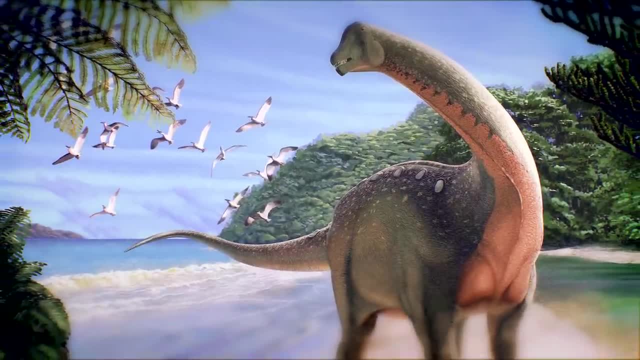 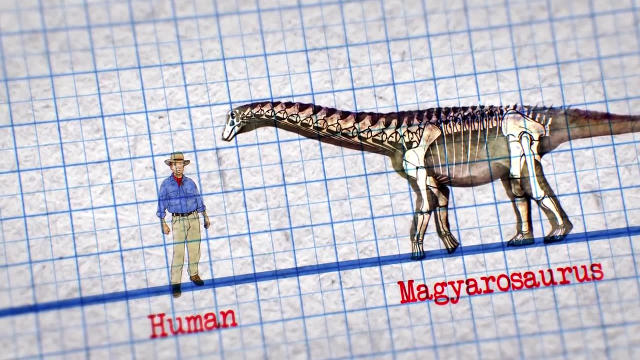 one that hadn't yet grown into a full-sized adult by the time of its death. But later study and analysis of its skeletal structure found this assumption to be wrong, confirming that these were in fact the bones of an adult titanosaur, just a truly tiny one. 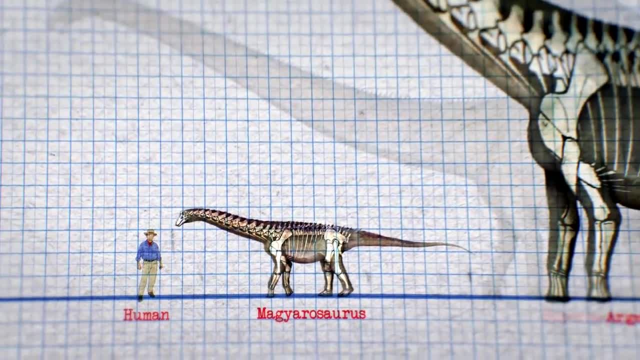 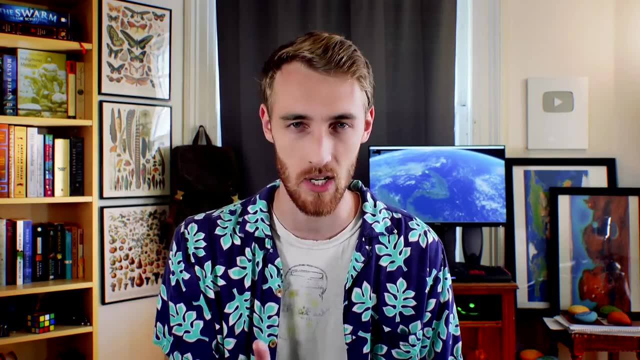 though no one could come up with a reason as to why this species was so stunted compared to other members of its clade. This didn't sit right with Nupška, however, who figured there must be a reason and explanation behind this species' less-than-impressive stature. 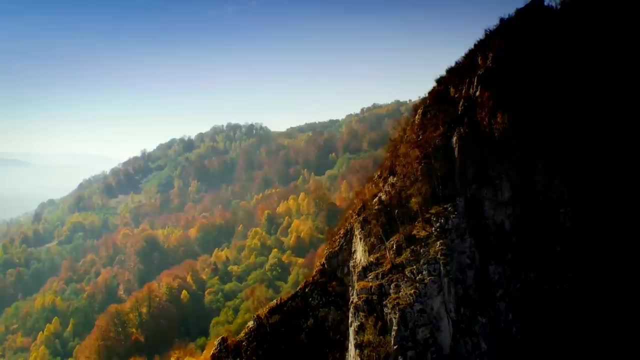 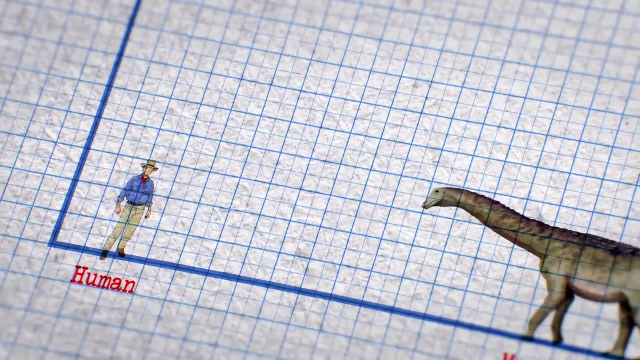 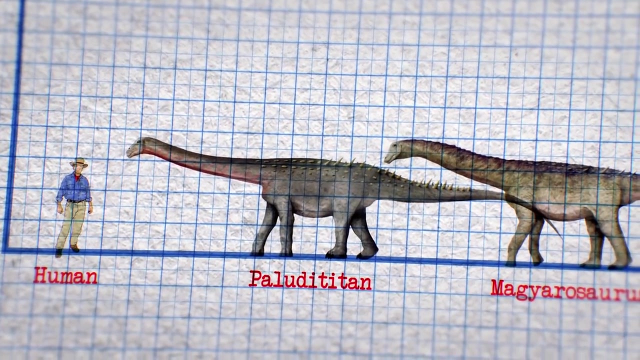 And as Nupška continued to dig, he only found more and more proof that something strange was happening here in the mountains of Transylvania. Another titanosaur uncovered at this site, Paludotitan, exhibited the same shortcomings, likely standing even shorter than Magyarosaurus, but perhaps a little longer from head to tail. 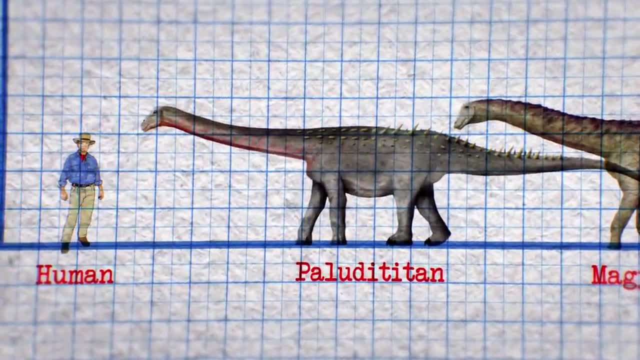 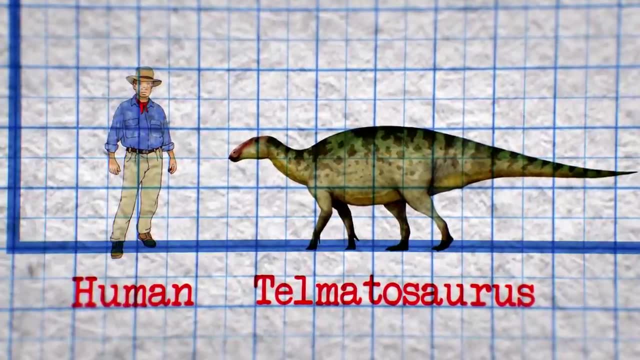 This trend extended beyond just the sauropods discovered, though, and later Nupška would describe the hadrosaur Telmatosaurus recovered from the same site, with a body that measured only three meters long, or less than half the length of your typical hadrosaur. 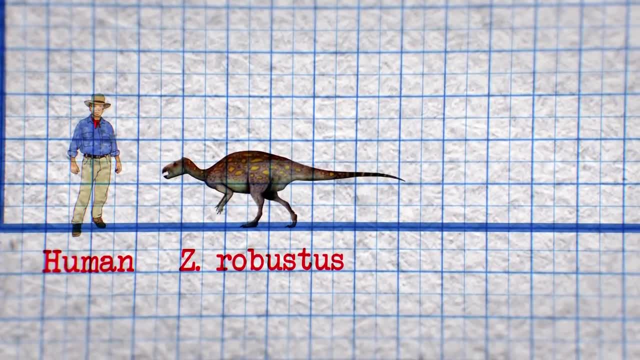 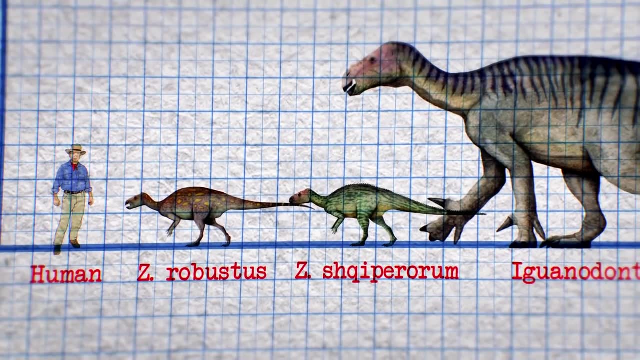 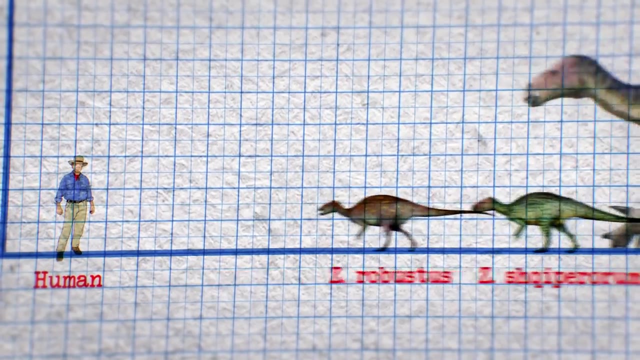 Two iguanodons found on site, Zalmoxis robustus and Zalmoxis schiquiparorum, both paled in comparison to their relatives, standing less than a meter tall, while other iguanodons found in surrounding areas stood over three meters tall. The same was also true for the 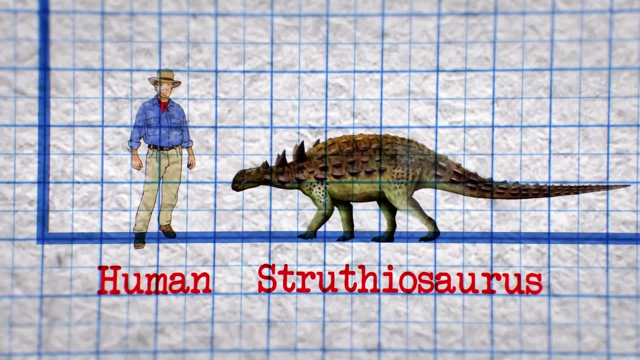 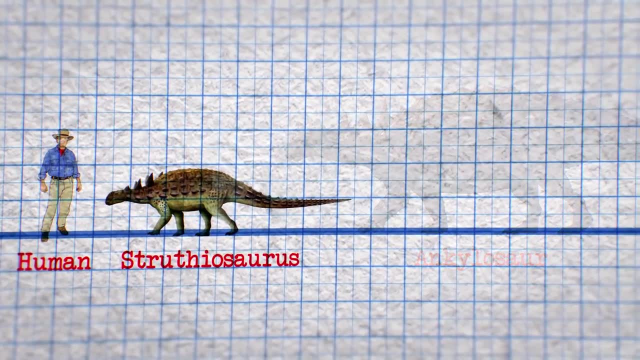 angiosaur, which was also found on the same site, but with a length of less than a meter, while the angiosaur found on site Struthiosaurus, which stood less than a meter tall, again less than half the height of angiosaurs observed elsewhere. Altogether, what Nupška found was that every 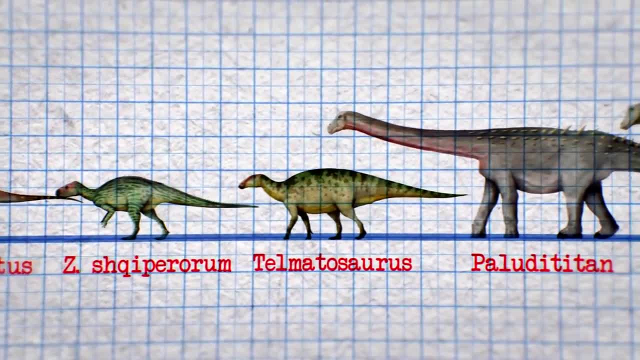 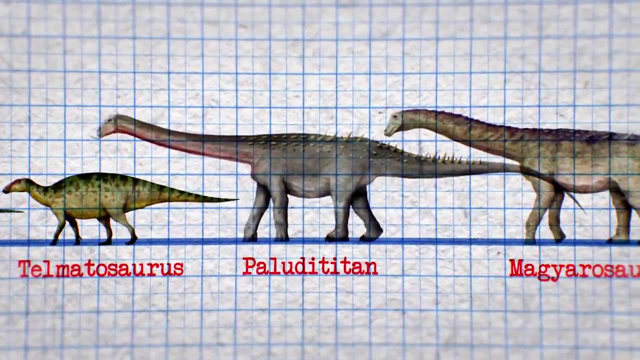 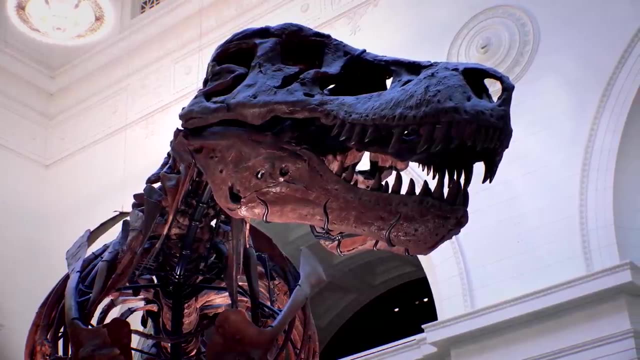 large herbivore uncovered at this site was seemingly affected in the same way, all severely reduced in size, and it was up to him to explain why. But Nupška was a smart man, and so, while most people in his field were more concerned with simply assembling what bones they 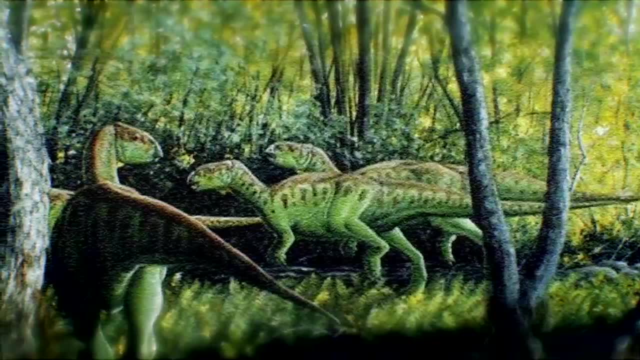 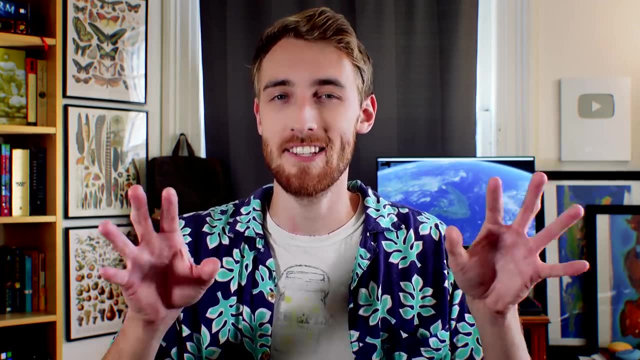 could uncover, he started to think about how these creatures would have actually lived and the factors that might have influenced their growth. Eventually, Nupška would come up with a simple idea that, despite being rejected initially, would go on to become. 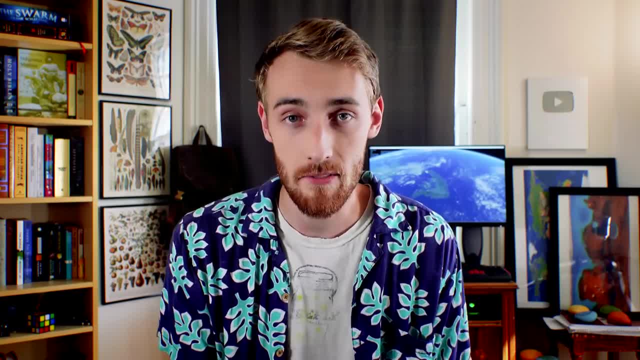 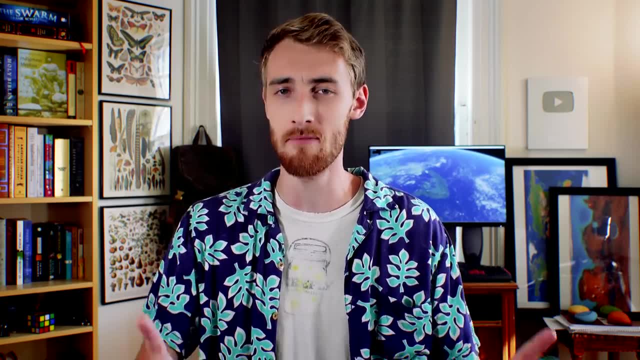 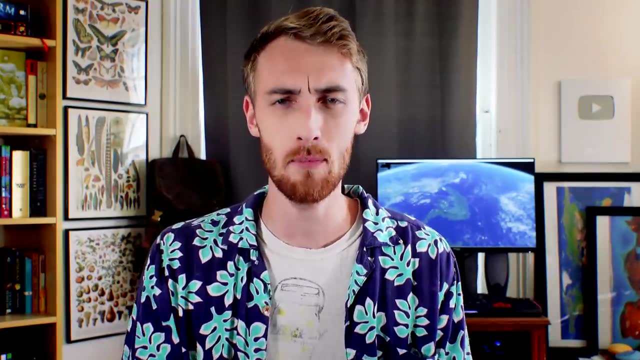 widely accepted within the scientific community. His line of thinking went like this: the only thing that could have caused such drastic shrinking across all animal groups must have been severe limitations of resources, like available food in the environment. But there also had to be a reason these animals didn't just abandon this food-scarce region. some external or environmental or even geographic feature that kept these animals from leaving for long enough that their physiology adapted to this scarcity? Hmm, okay. so what kind of environment do we know of that both produces less food and also geographically isolates its inhabitants? 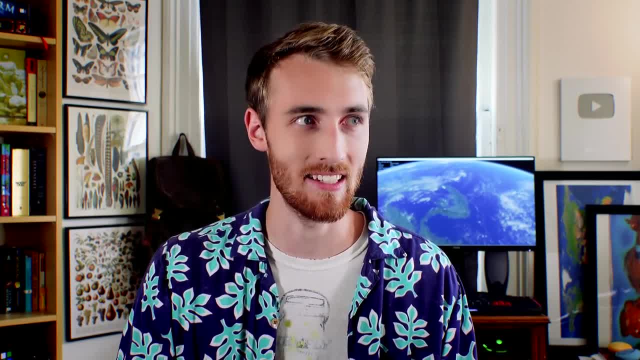 Well, I don't know about you, but to me that sounds exactly like an island. and well, Nupška thought the very same thing. Nupška thought the very same thing. Well, Nupška thought the very. 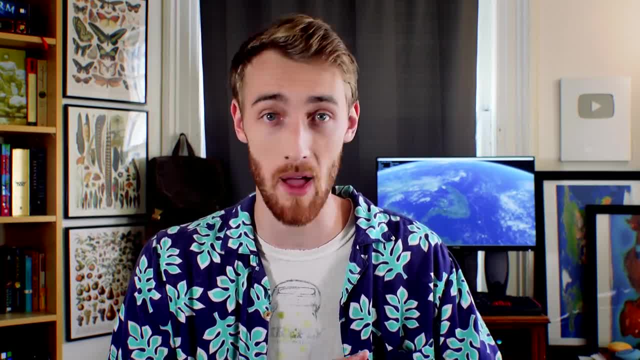 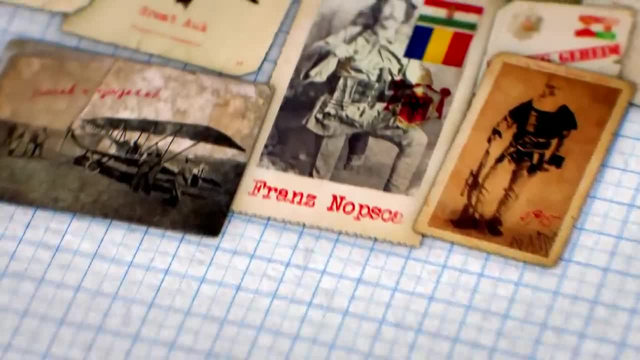 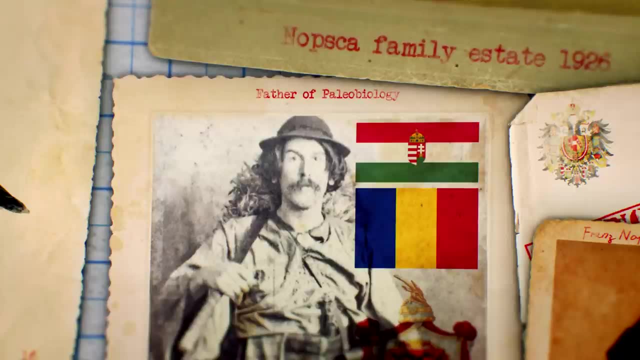 same thing In the process, becoming the first person to ever describe the now well-established theory of island dwarfism. For this, Franz Nupška is considered to be the founding father for the field of paleobiology, and his ideas continue to influence how we think about island. 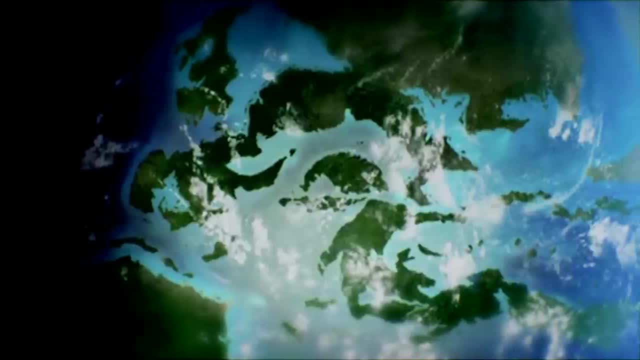 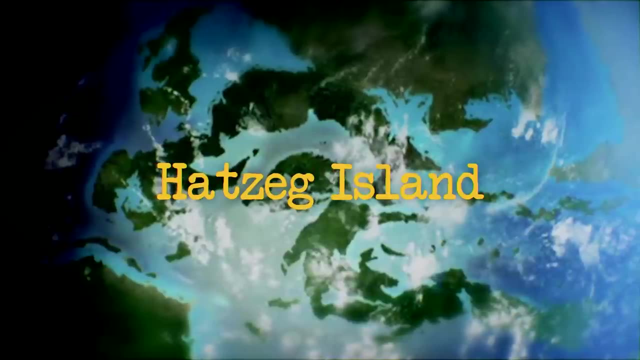 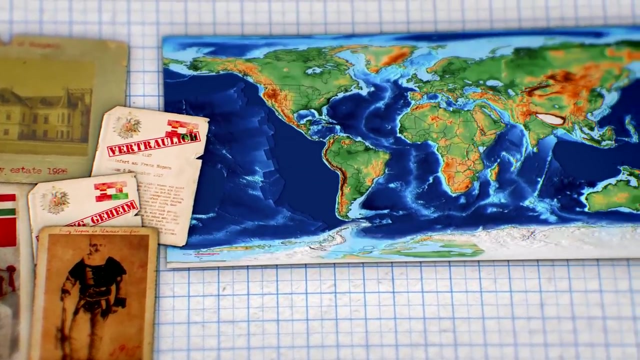 ecosystems to this very day. For the area in which these fossils were discovered, this theoretical ancient island was given the name Hatsag Island, Based on the age of the specimens uncovered, Hatsag Island must have existed around 70 million years ago, which is a little unfortunate because the map I typically use to travel back in time with 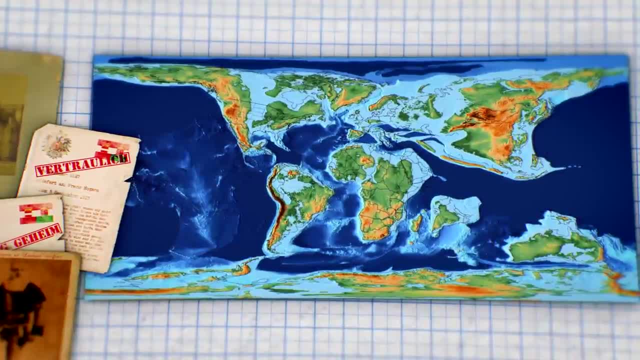 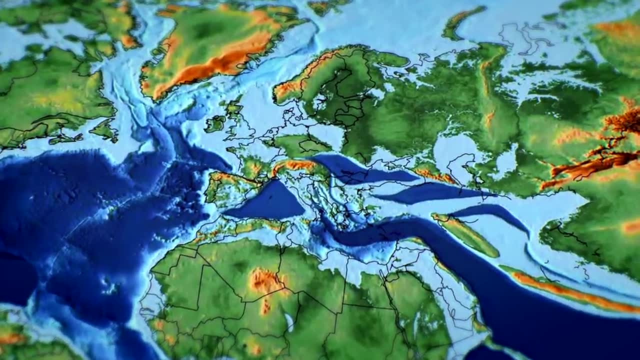 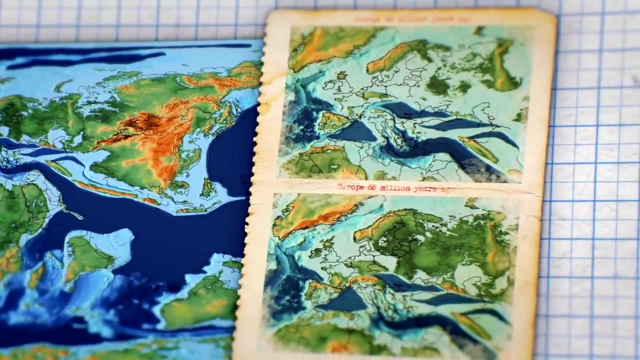 only has frames representing 80 million years ago and 66 million years ago, both of which are either too early or too late in time to accurately show the island. However, at the very least, what these two maps do show us is that, throughout this time, higher sea levels like the one in the 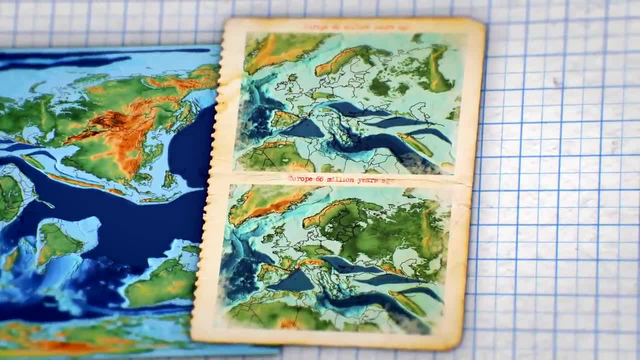 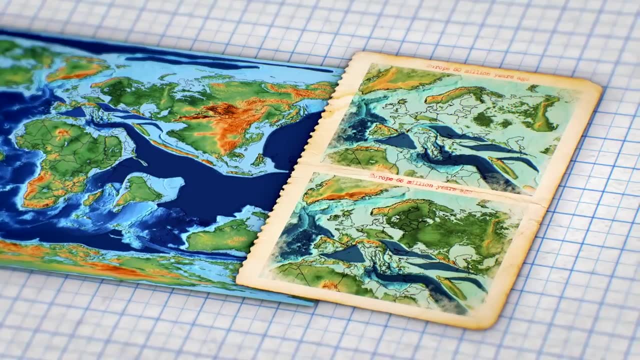 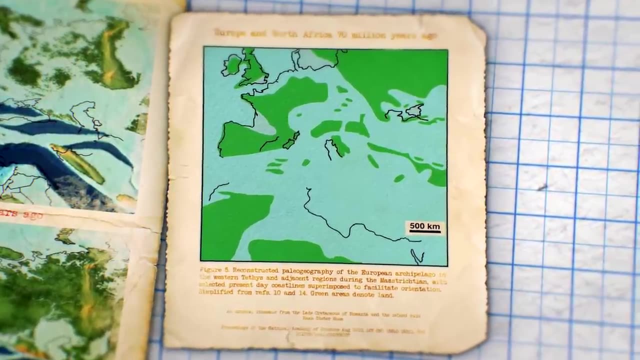 middle left most of Europe underwater as part of the Tethys Sea, supporting the concept that what is now inland Europe could at this time have been surrounded by the ocean. But to see any more we'll have to look at later geological recreations of this region, like this one published in 2010.. 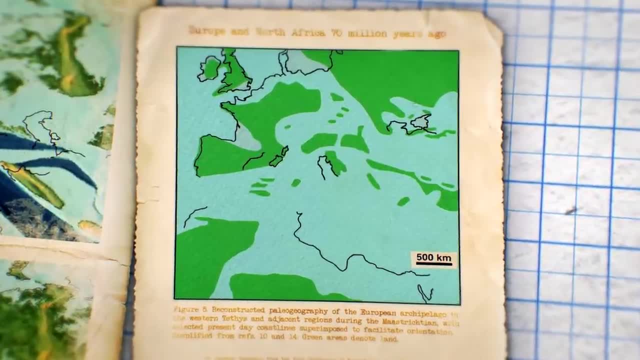 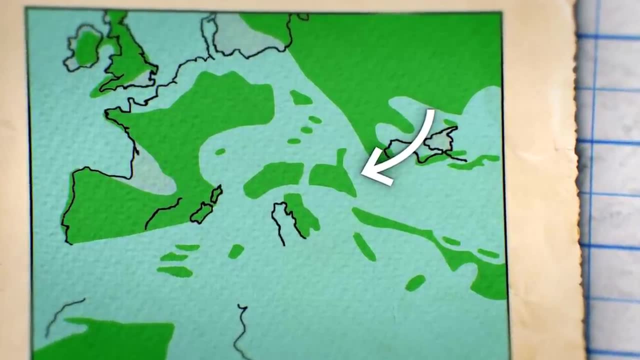 Doing this, we'll find that well, Nupška was right. A portion of what would become the Transylvanian Alps managed to have peaked above the heightened sea levels of the time to produce an island measuring approximately 1.5 million years old. This is a very good example of how 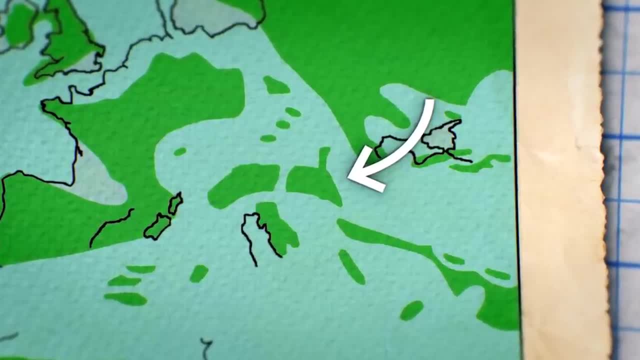 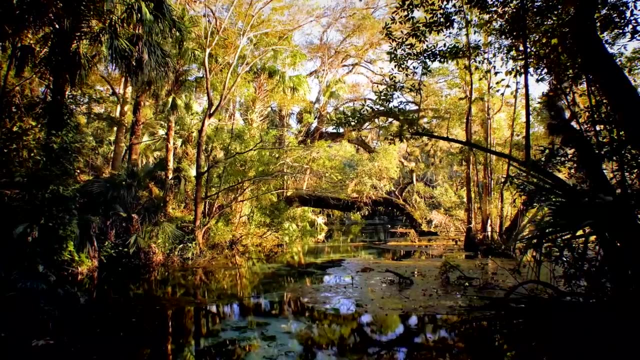 the Alps were built in the early 20th century. The Alps were built approximately 80,000 square kilometers, or roughly the size of Ireland. Plant fossils recovered from this site show that mostly tropical plants grew here, likely fed by a seasonal monsoon, creating a warm and swampy. 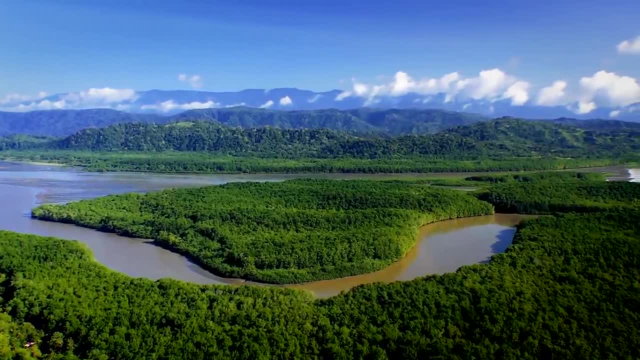 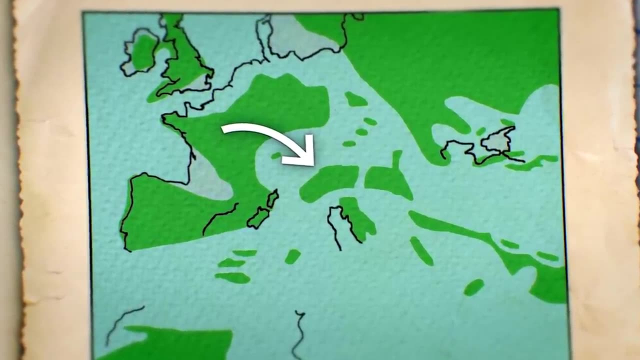 environment quite different from the temperate climate of Romania today. To the west of Haceg Island, we can see the mountains that would eventually become the Alps also stood above the ocean to form a slightly larger island, while the Dinaric Alps to the south built. 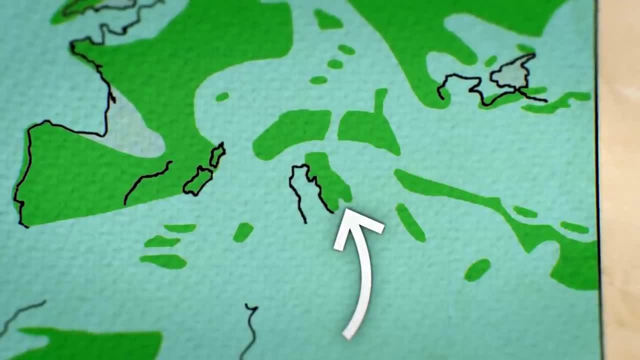 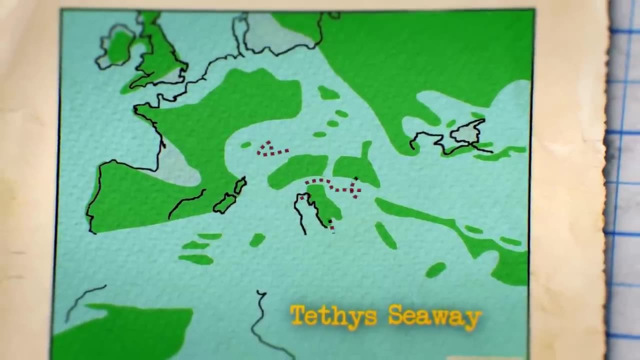 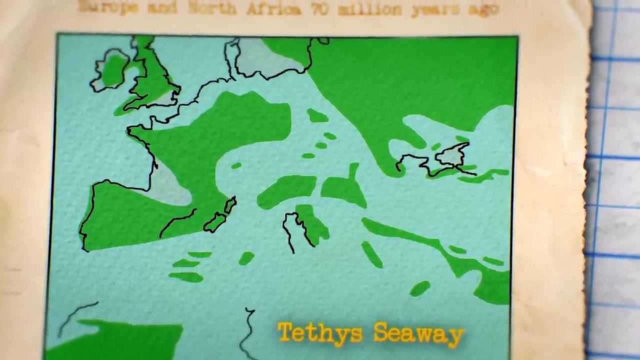 up a third, slightly smaller island, all together forming a significant archipelago smack dab in the middle of the Tethys Seaway that all likely would have regularly traded species with one another. Looking beyond this cluster of mountainous islands, we can see that the partial submerging 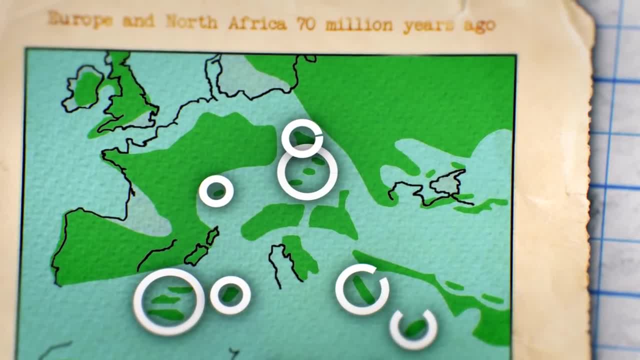 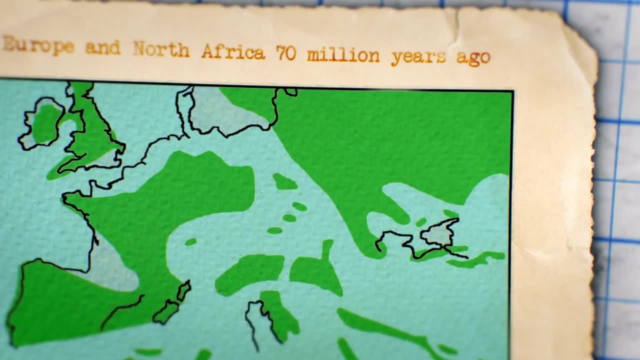 of Europe produced numerous other small islands across the continental shelf, though this wasn't enough to put what's now Eastern Europe beneath the water which stood at this time as the landmass of Phenocermatia- Phenocermatia, which I promise is a real name and not one I just made up. 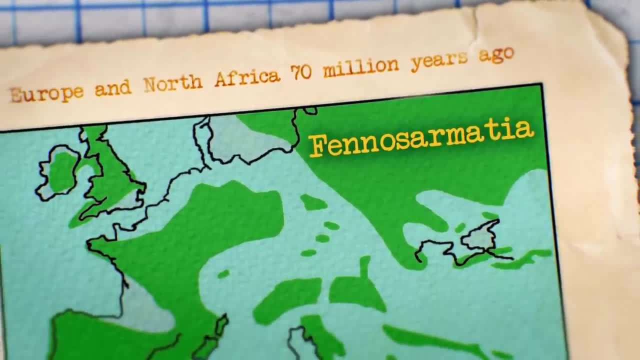 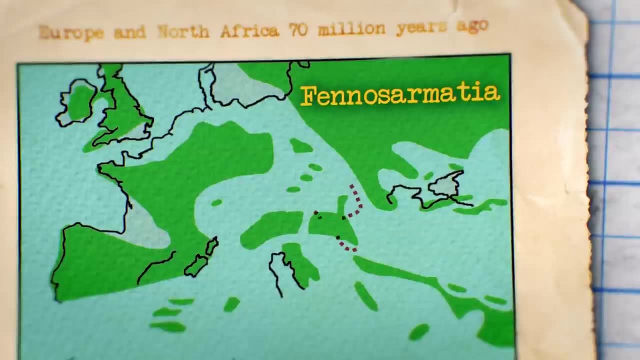 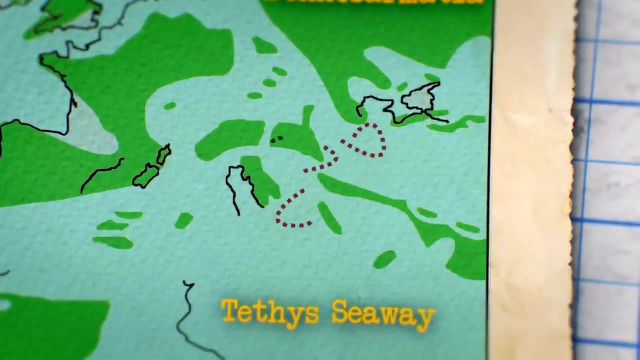 At only around 200 kilometers away from Haceg, Phenocermatia likely would have been the primary donor of mainland species that would eventually come to inhabit the island. Other sources of species influx could have been from the connected Balkan Anatolian highlands, which sat even closer. 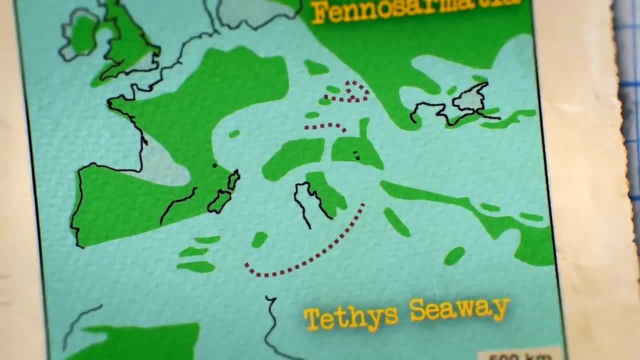 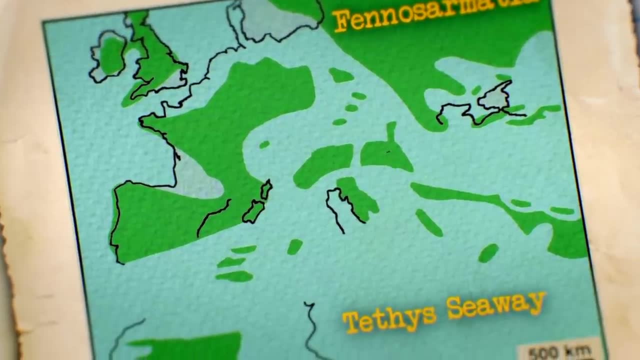 to Haceg, as well as the connected lands of what would become Spain and France, which at this time stood as the region of the island. The island was also known as the island of the island, which was the region's largest island. However, the raised sea levels also pushed the northern coast of Africa. 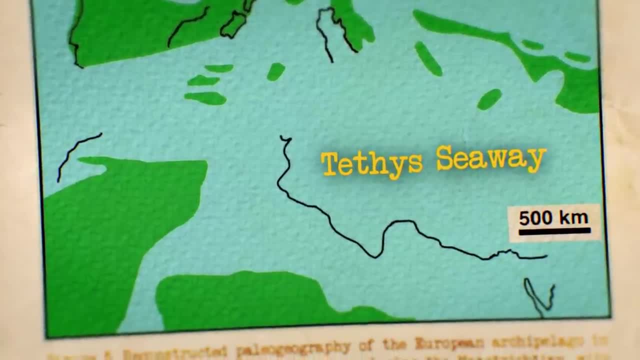 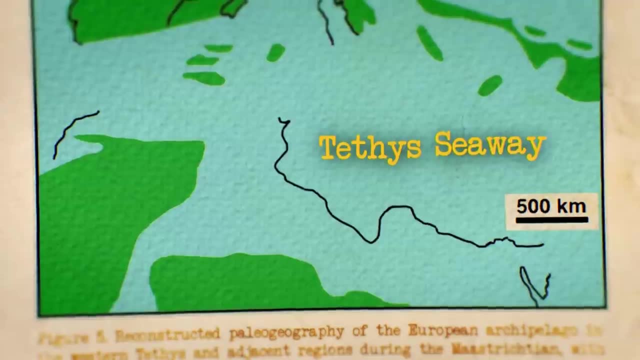 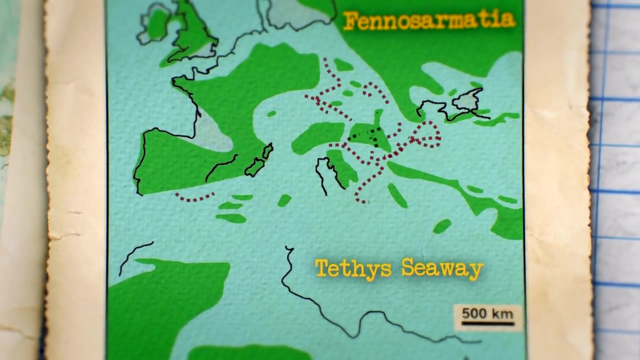 much further back, making it unlikely that Haceg Island would receive many colonization efforts from the African fauna of the time. Overall, Haceg Island's position within this cluttered sea not only meant that it stood to receive genetic influx from multiple sites, but also that it wasn't only 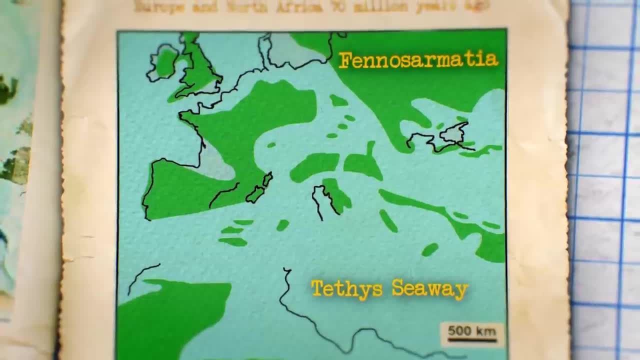 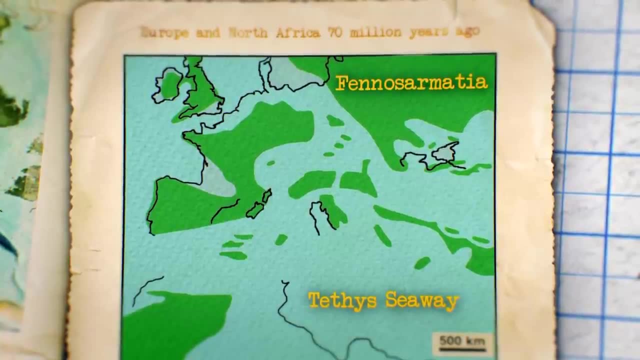 accessible to flying creatures of the time, and by moving from island to island, larger terrestrial animals were also capable of reaching its shores, explaining how something as huge as a titanosaur managed to get here in the first place. But if it was easier for mainland herbivores to find that, 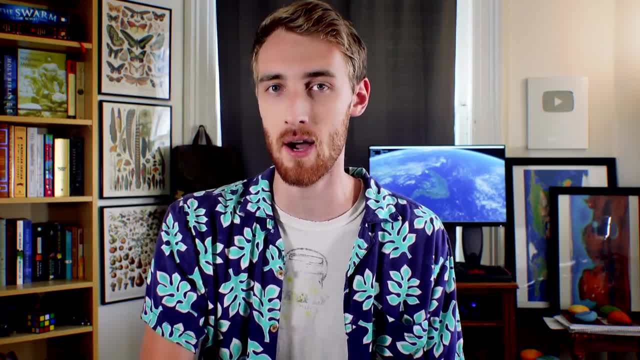 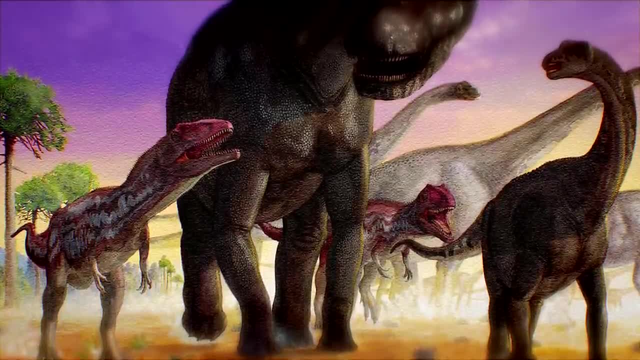 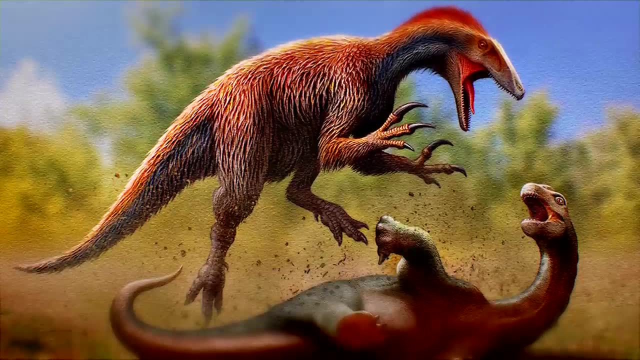 also means other large animals like the carnivorous theropods could find their way here as well. The only problem was that when these predators arrived, they found their usual prey that had once been large enough to provide a good meal had shrunk down into what can only be described as a snack or an. 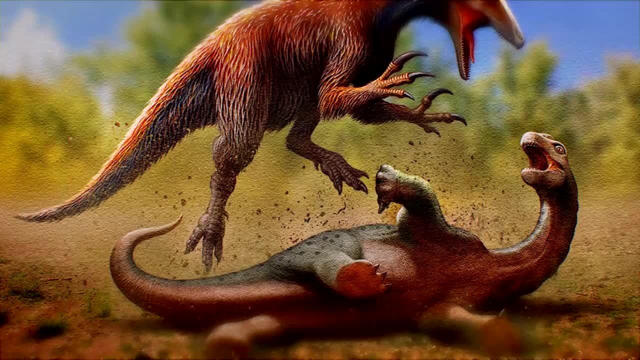 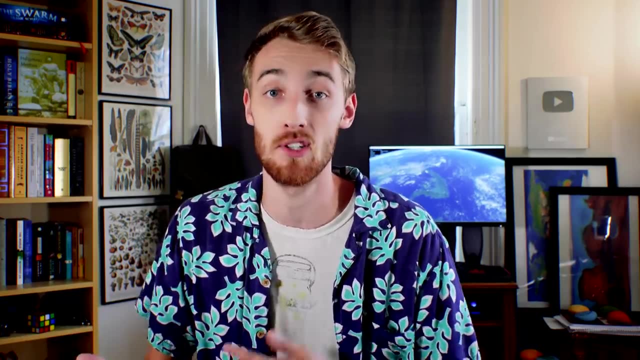 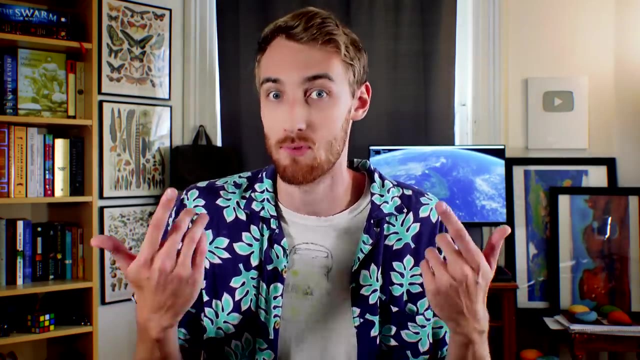 animal food, In other words, incoming theropods, also found a food-limited environment, And so just as the herbivores adapted to less plentiful grazing by growing smaller, so too did the carnivores adapt to the severely reduced size of their prey, by also growing smaller. From mainland species like 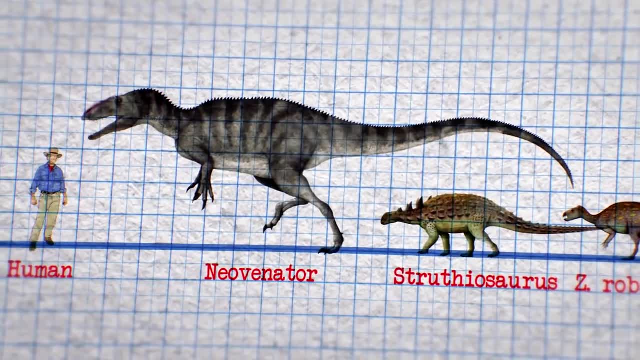 Neovinotaur which stood up to 2.5 meters tall. Franz Nobschke found that Haceg Island had produced Heptaestaeornis which stood just over 2.5 meters tall, and that Haceg Island had produced Heptaestaeornis. 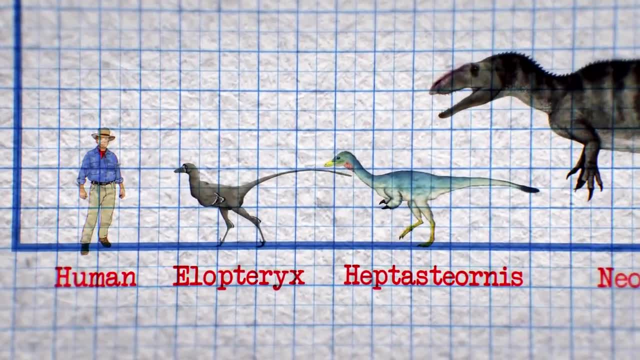 which stood just over 2.5 meters tall, and that Haceg Island had produced Heptaestaeornis, which stood just over 1.5 meters, and Elopdorix, which came in at only 1.2 meters tall. At sizes this small, not only would 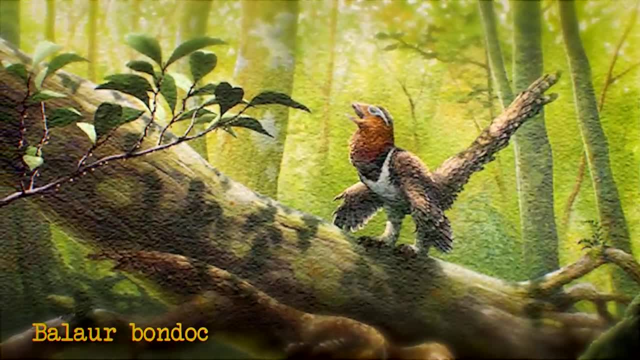 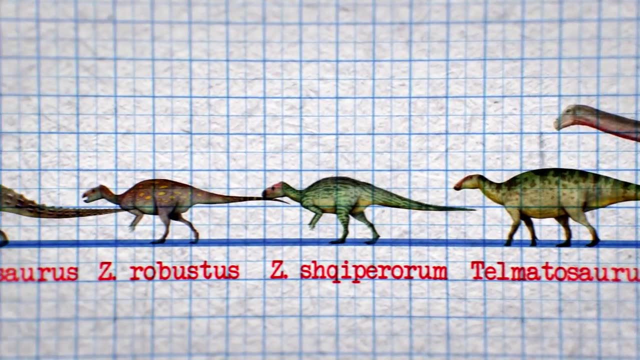 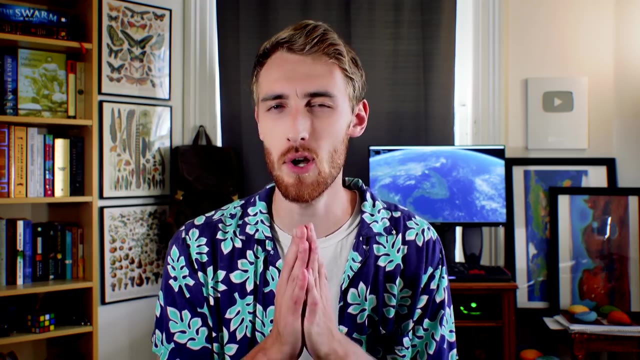 these former terrifying creatures have been well adorable, but they also would have been dwarfed by the very animals they used to hunt, forcing them to feed on the much smaller creatures inhabiting the island, causing theropods to lose their status as apex predators here. But if you know, 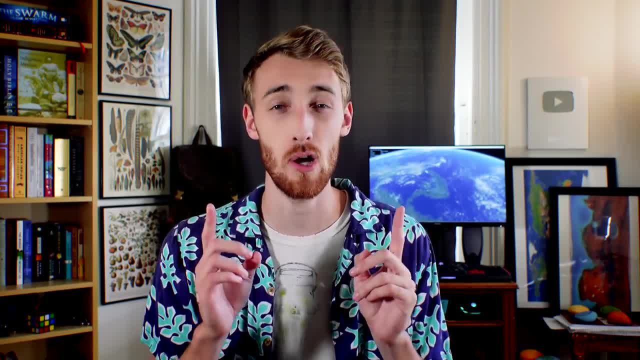 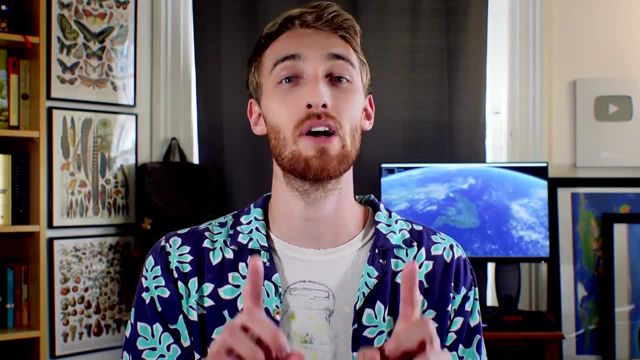 anything about ecology, then you know this would only leave a hole in the Haceg community or, better yet, a niche left unfilled, And whenever this happens, it's only a matter of time before something else comes along to take its place, Before we can get. 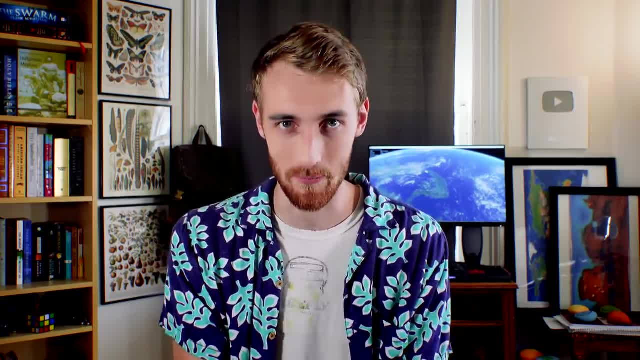 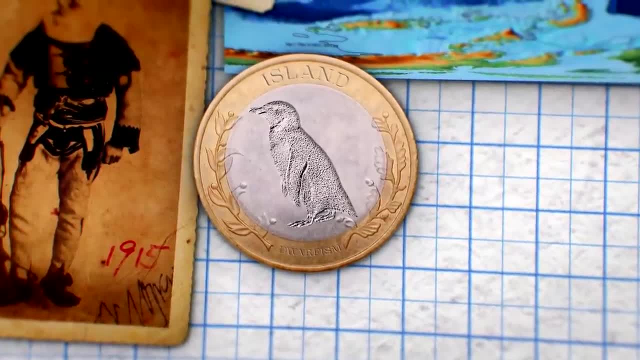 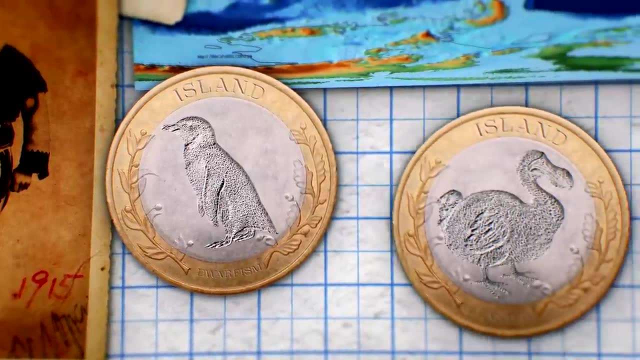 into it, though we need to do a little bit of review. If you've really been paying attention to these past two videos, you know that island dwarfism is only one side of the coin that animals flip when coming to a new island, with the other side of this coin being a trait known as island. 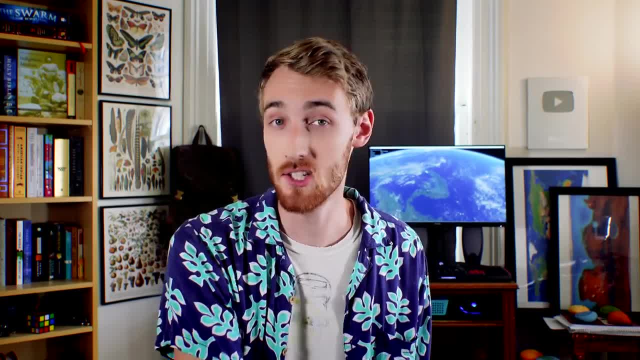 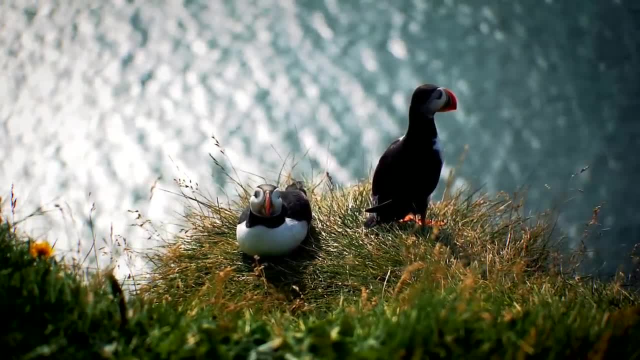 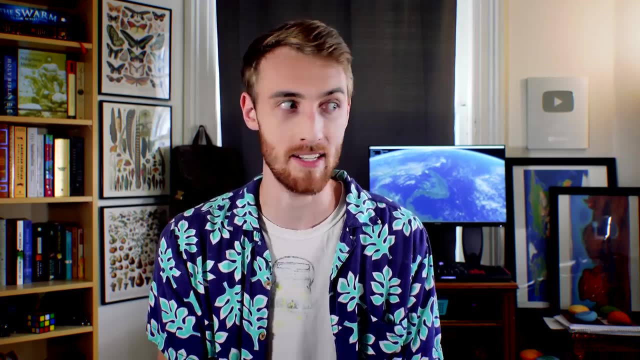 gigantism. This tends to happen when a continental animal starts off small. In the last two videos, this meant looking at birds which are by nature small, in exchange for the ability to fly. But during the time of Haceg Island, birds had yet to fully evolve and instead the skies were ruled by 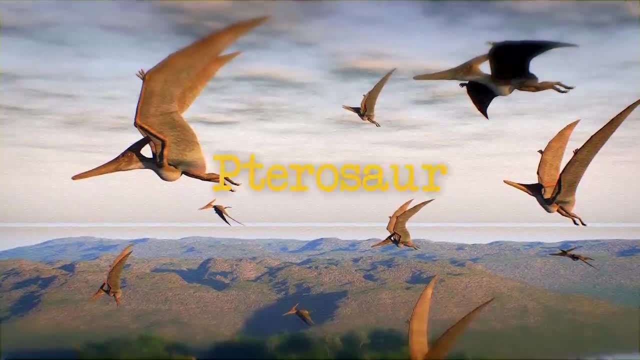 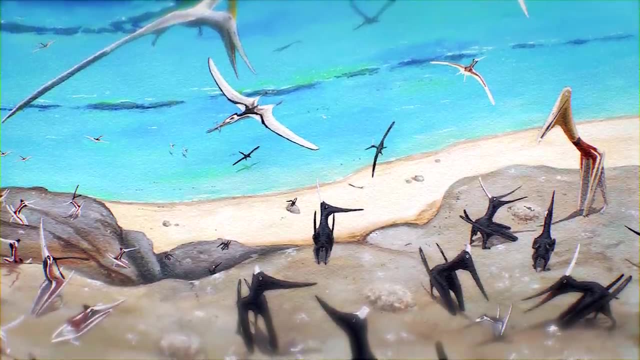 a different creature. This was the age of the pterosaur, and much in the same way that birds today seek out and thrive in every scrap of land raised above the water, 70 million years ago this role belonged to these winged lizards. Haceg Island was no different. 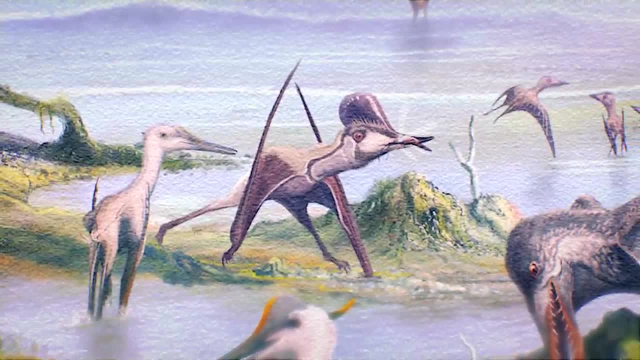 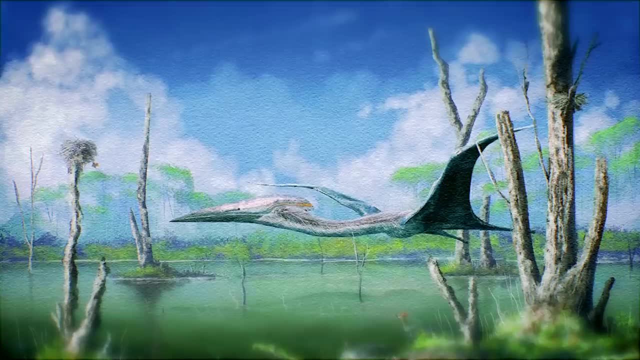 and likely thousands of years. before the first titanosaurs or theropods made their way here, pterosaurs must have flocked to its shores and nested here for good. Those that did found a bountiful place, at least from their perspective, giving them an early advantage here. that over 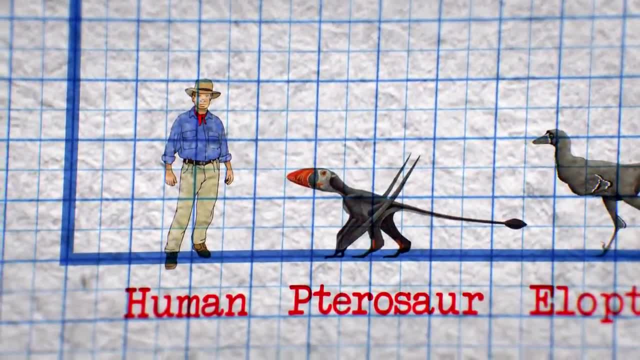 time transformed these fortunate pterosaurs from a small and compact half meter tall into a small and compact half-meter-tall pterosaur, and from that small and compact half-meter-tall into a small and compact half-meter-tall pterosaur, and from that small and compact half-meter-tall 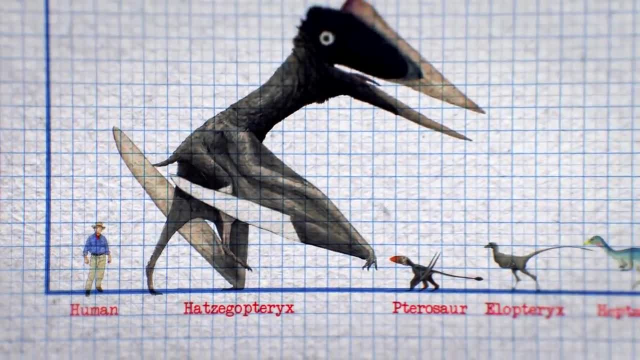 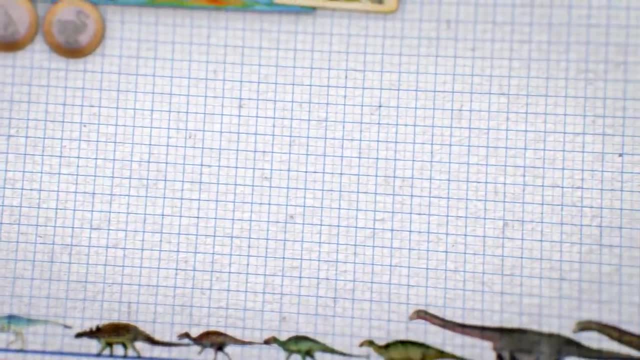 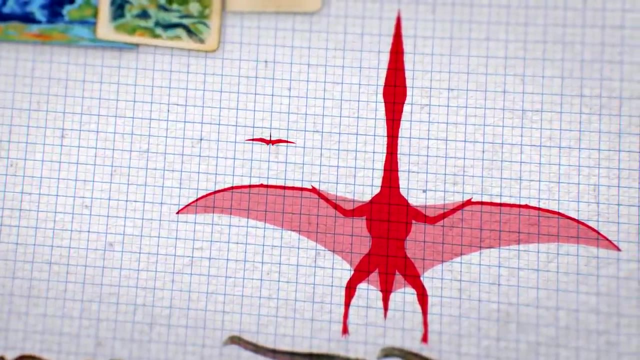 to the incredible Hatzegopteryx, which loomed up to 6 meters tall, But well okay, these are flying creatures after all, so maybe a better metric to demonstrate their amazing size would be their wingspan, which could reach up to 12 meters long, compared to only a single meter typical pterosaurs. 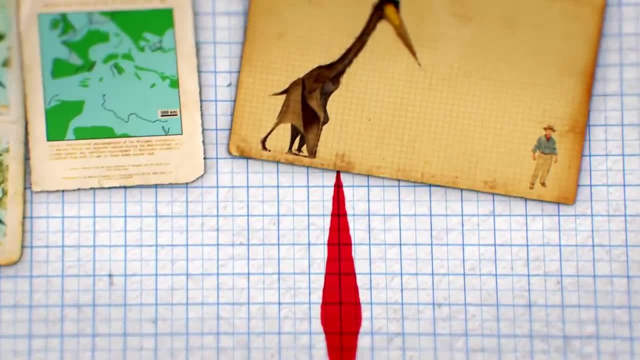 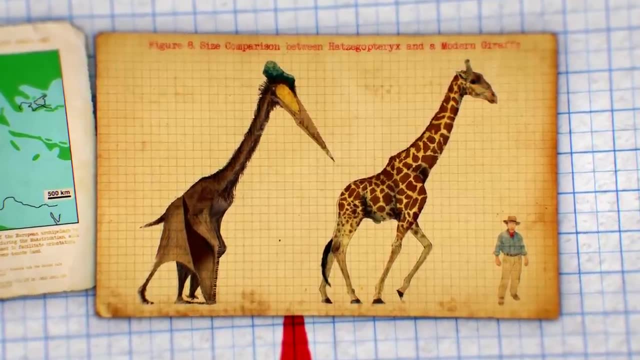 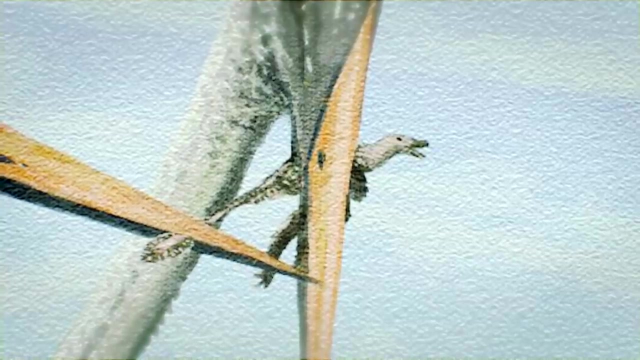 grew to. With these dimensions, Hatzegopteryx would have almost resembled a giraffe in terms of height and shape, except with the addition of a massive beak meant for snapping up prey, not much smaller than an average human. This made Hatzegopteryx by far the largest. 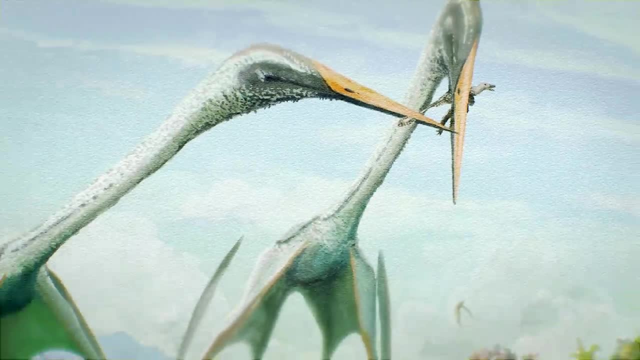 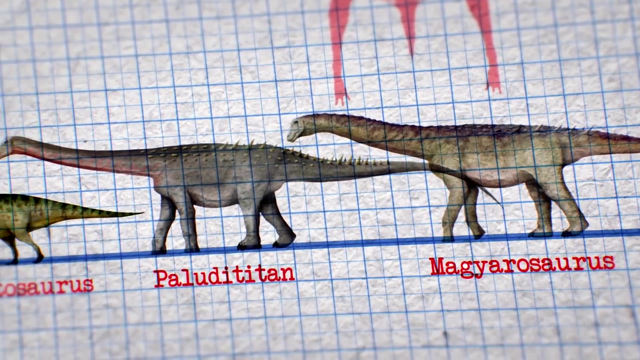 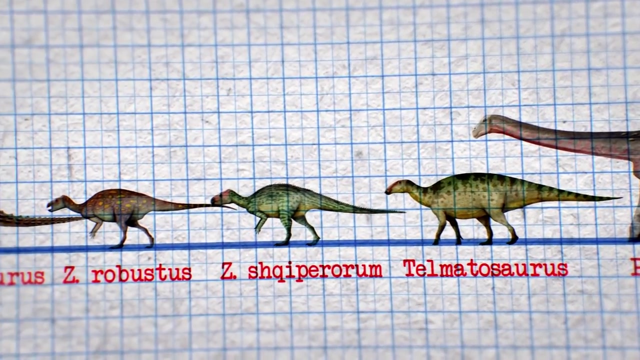 predatory animal native to this island environment, giving it the dominant carnivorous role and the title of apex predator. When looked at as a whole, the animal community of Hatzeg Island first described by Franz Nobschke, looks like a typical dinosaur hierarchy, turned upside down. 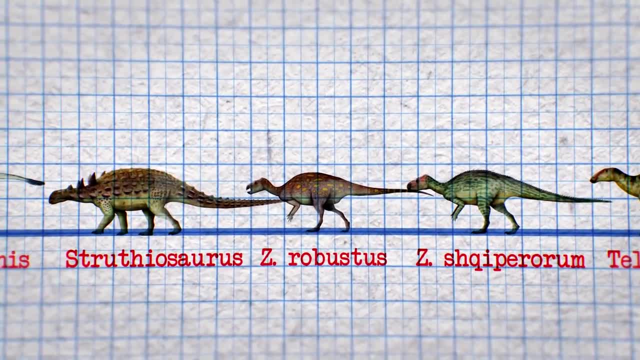 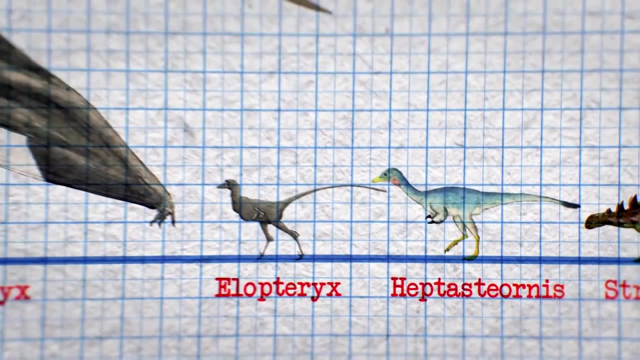 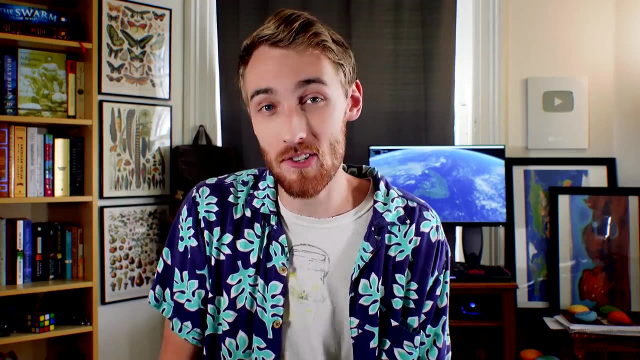 where the typical giants had become stunted beyond recognition. The most feared mainland predators were reduced to scavenging for low-tier prey, and a normally tiny creature was given an evolutionary head start, allowing it to rule as king of this domain. In a bigger sense, what the fossils discovered at this site have revealed to us is that evolution 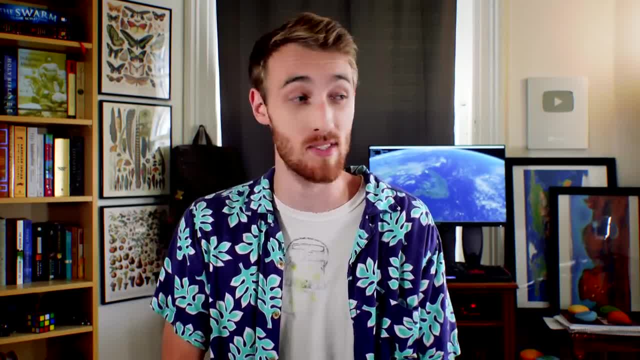 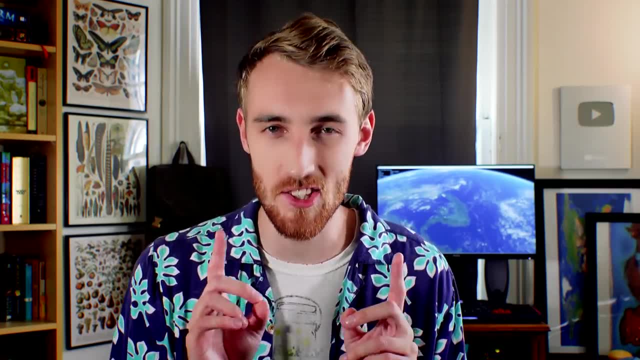 is always taking place, and the factors that influenced life 70 million years ago are the same factors that influence us now. Hatzeg Island serves as just a single example, a microcosm representing the millions of possible lifeforms that could have existed.